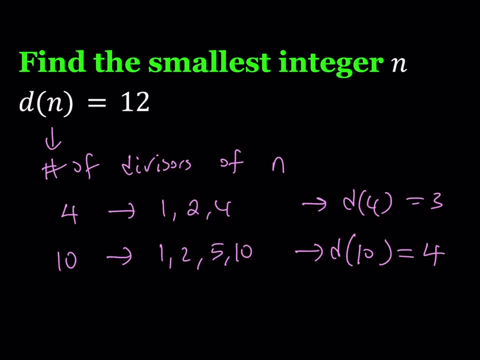 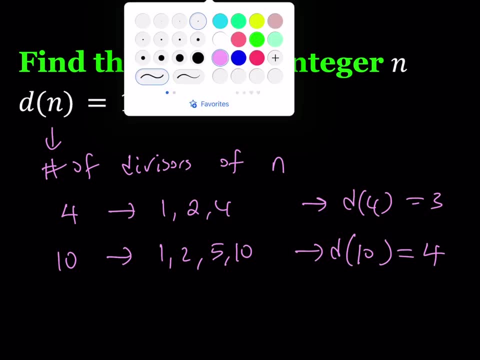 without listing them all, because listing is not practical. what if they gave you 25 million? are you going to list all the divisors? i don't think so. right, i mean, you can try it, but you know that's going to take forever. great, so let's take a look at an example. for example: um, how about four? let's. 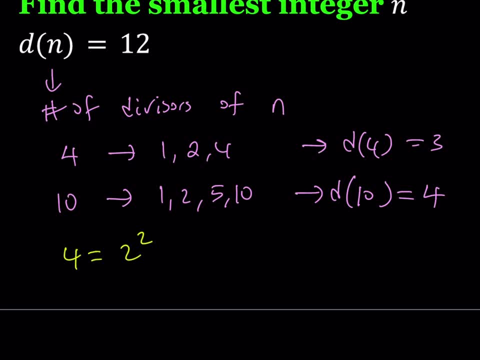 take a look at four. well, four can be written as two to the second power. that means any divisor of two to the second power needs to be in this form: two to the power zero, two to the power one or two to the power two. so that gives you three divisors, easy right. so how do you get there? let's do look. 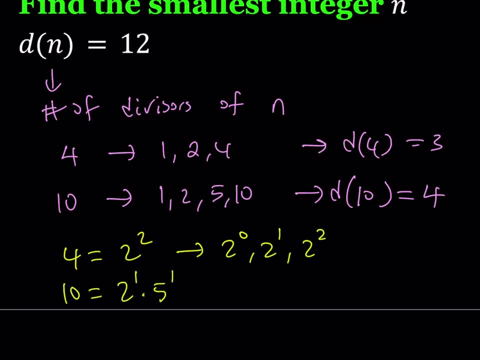 at ten. well, ten can be written as two to the first times, five to the first and, as you know, any divisor of ten is going to contain two or five, or both or none of them. so it could be like two to the power zero, two to the power one with five to the. 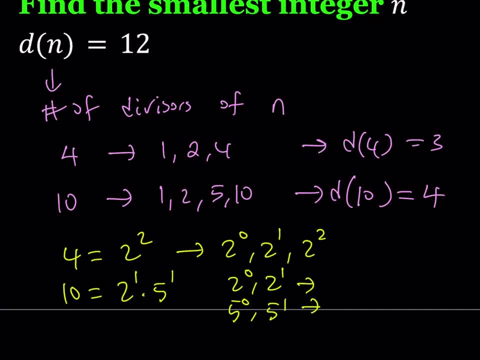 power zero five to the power one. we have two lists and we we have to pick an integer from each list. that gives us two times two, which is four options. now here's where this comes from. you look at the exponents in the prime factorization and increase each one by one and 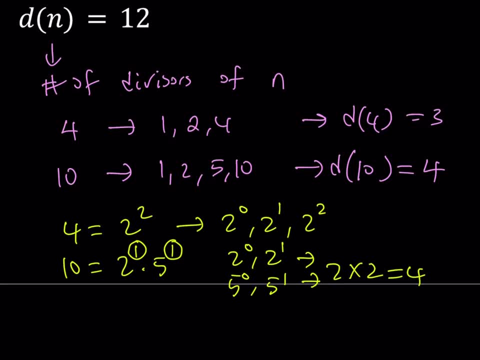 then you get the number of divisors. so in the case of four, since there's only one prime, you take the largest power, which is second power, and increase by one and you get the three, which is d, of four, and in this case it's one plus one, multiplied by one plus one. and these ones come from here, okay. 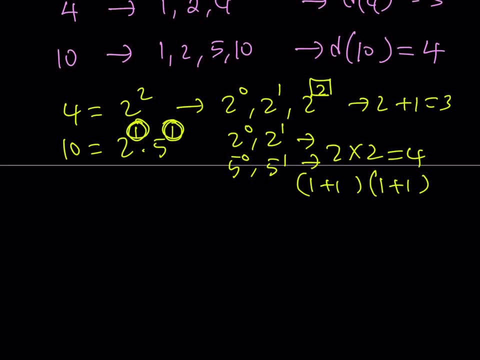 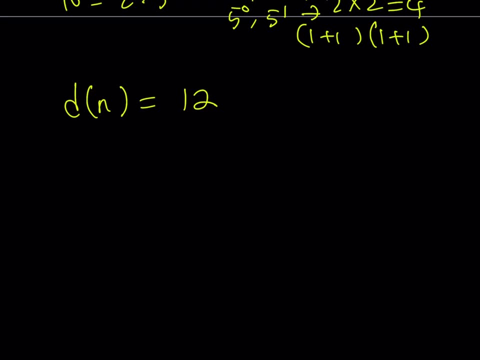 great. so that's how we find the number of divisors of an integer. now here's the question: how do you reverse this process? well, you look at the number and you factor it. so we're going to go ahead and factor 12.. we're going to start by factoring 12 and then looking at different ways to factor it. 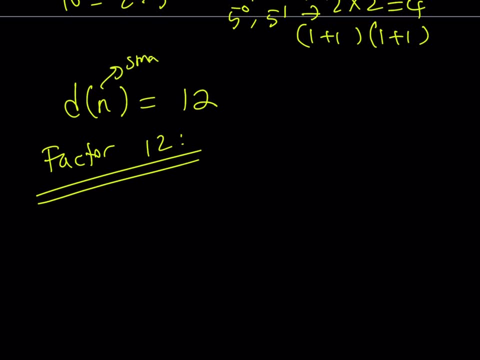 and remember, our goal is to find the smallest, and that satisfies this great. so 12 can be factored in a couple different ways. for example, 1 times 12, 2 times 6 or 3 times 4.. this also shows you that d of 12 is 6, but we don't really care about that. 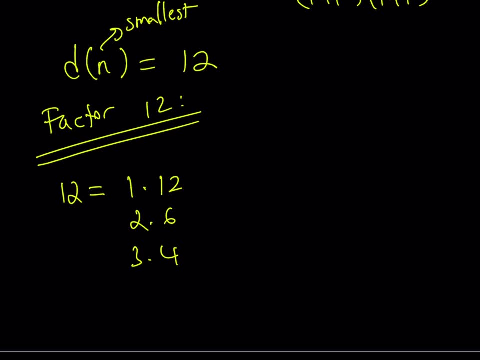 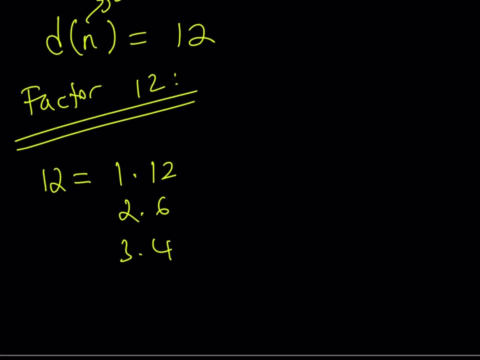 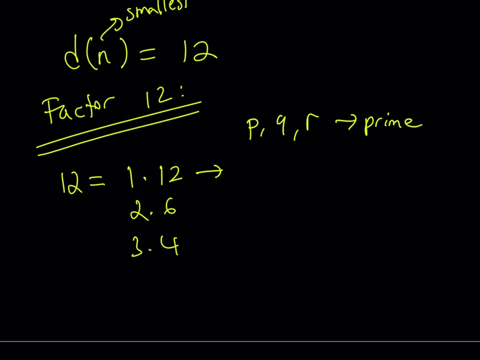 right now. now, what does 1 times 12 mean? well, it just means that the when you increase the exponents by 1, you get 1 and 12.. so if you decrease these numbers by 1, you get the exponents. so suppose p, q, r are prime numbers and we can write this as p to the: 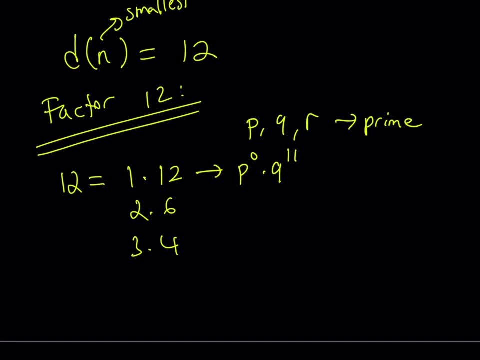 power 0 times q to the power 11.. think about this number for a minute. you have something like p to the power 0, which doesn't really matter because it's 1, or you have something like 2 to the power 11, for example. right well, how would you find the number of divisors of this number? 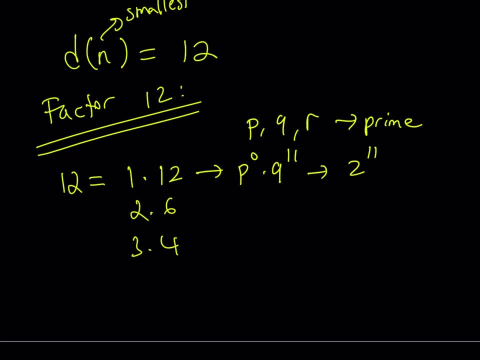 you're just going to take the exponent and increase by 1 and that's going to give you 12.. that's what i'm talking about. so that's how we reverse the process. but notice that 2 to power 11 is 2048. what is that the smallest number? i don't think. so let's go and take a look at 2 times 6.. okay, 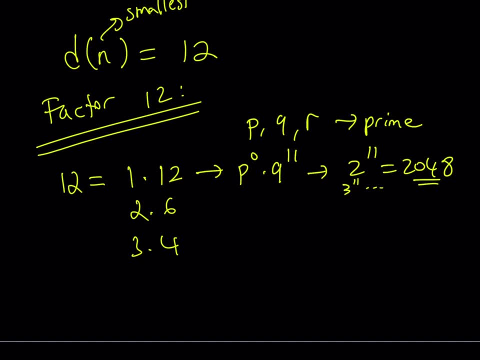 well, obviously, if you used 3 to the power 11, that's going to be even larger, so don't even go there. 2 to the power 6. now how do you reverse the process? so i know d of n. i need to find n. you take the numbers, that are the factors, decrease each one by one and use them as exponents: p, q, r. 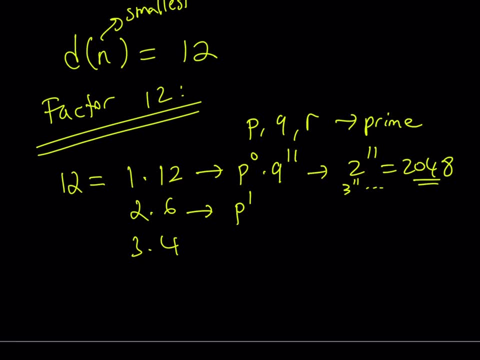 are the basis right. so i have something like p to the first and q to the fifth, because 2 and 6 are one more than one and five right. but this gives you a bunch of options. for example, i could do two to the first times, three to the fifth, or i can do three to the. 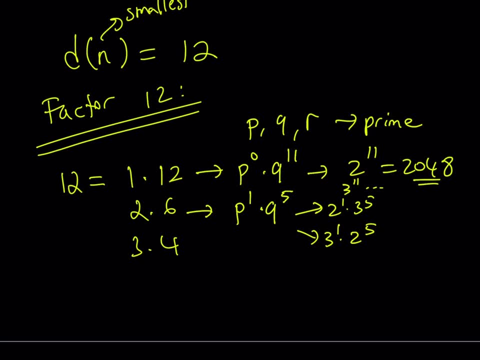 first, with two to the fifth. and here's an important fact: if you use the smaller prime with a larger exponent, it's better because your number will be smaller. for example, take a look at this one: this is 243 times 2, which is 486. that's a three digit number, obviously better than 2048. 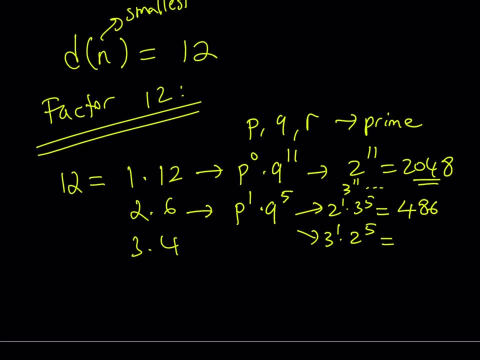 but can we improve on this? and we can. 2 to the fifth times 3 is going to be 96, and there you go. huge improvement, right. but are we going to stop here? no, because maybe three times four is going to give us something better. so we have to keep looking until we're sure that there is no better. 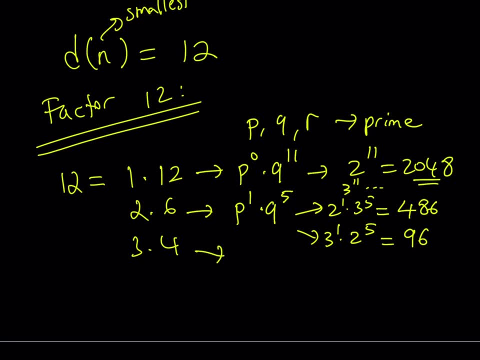 way to do it. so three times four can be broken down as p to the second times q to the third, and we're going to be looking at different options how this works out so i can use: remember we decrease by each number by one to get the exponent. but now i'm going to replace p and q with primes. 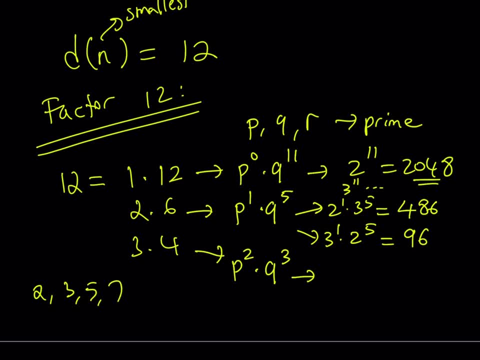 and remember our list of primes: two, three, five, seven. you don't really have to go far out because obviously if you go to 11, 13, they're going to give you very large results. so we have to stay. you know, somewhere here, maybe two, three, five at most. so let's use two to the second, three to the 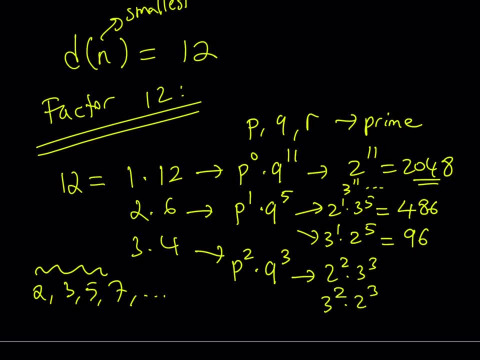 third- but remember we talked about this- this is going to give you something better. let's check it out four times: 27 is 108. uh, oh, it's even worse than 96. so i don't want that. i don't want any of them so far, but this one is going to give you 72, and it's even better. here's the million dollar. 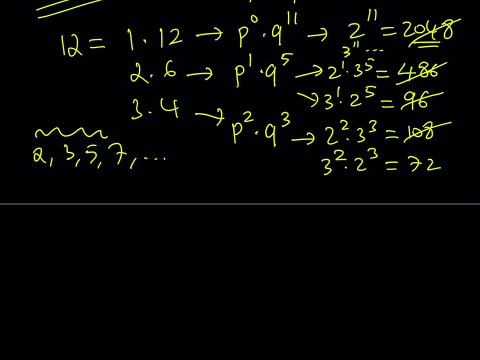 question: can we improve on this and get something smaller than 72? if that's the case, we have an answer. if that's not the case, then 72 is the answer. so let's take a look. and so the question is: can we find a smaller number with 12 divisors? and the answer is yes, but you have to think. 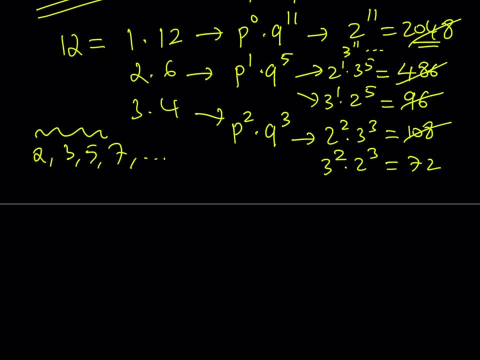 outside the box a little bit. instead of using two factors, we must use three factors. why? because distributing the 12 over more exponents is going to keep our number smaller because, remember, the base is not, it doesn't make a huge difference, but the exponents make a huge difference, because exponents are powerful. okay, you know what i'm talking about. 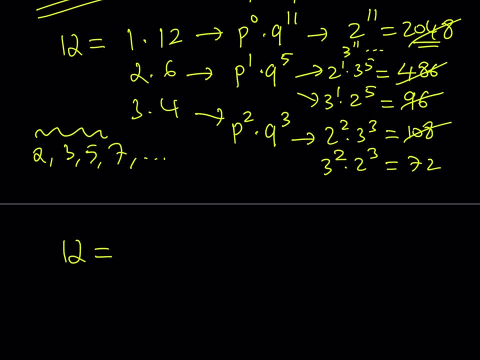 right, powers and powerful, great. so how can i do 12.. one times one times 12? no, i don't want to use one, because that just indicates zero power. so i want to do two times two times three, and this is just awesome. you'll see in a little bit why. okay, this indicates p to the power one. 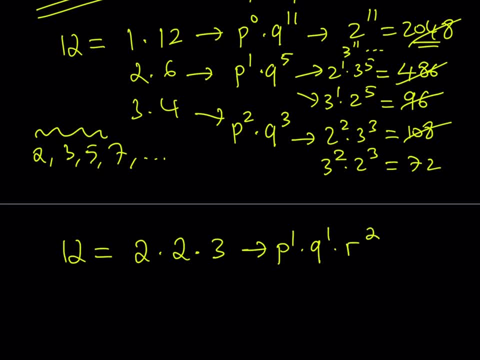 q to the power one and r to the power two. awesome. why is this good? because we're keeping the exponent real small as opposed to fifth. third, we're using first and second powers, so hopefully it's going to give us something nicer. let's test it out. well, since pq and r are distinct primes, i